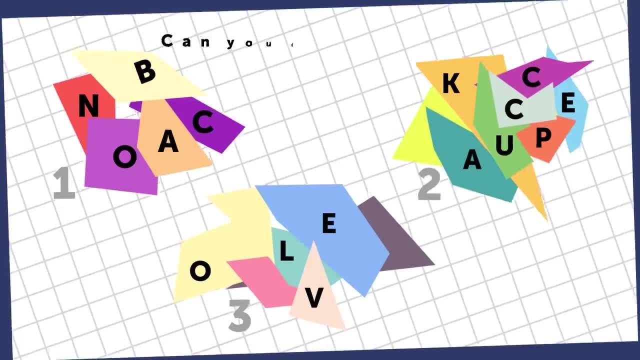 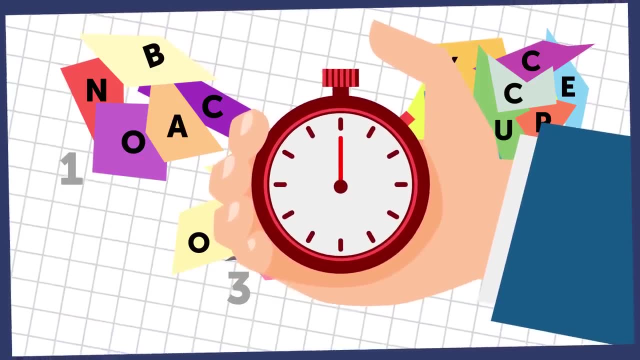 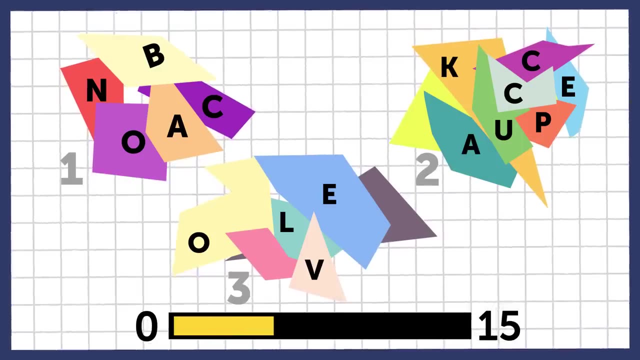 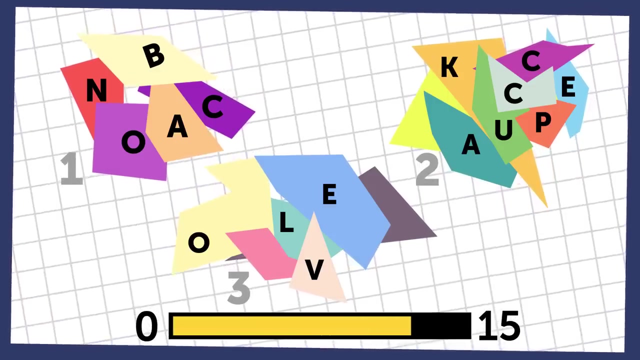 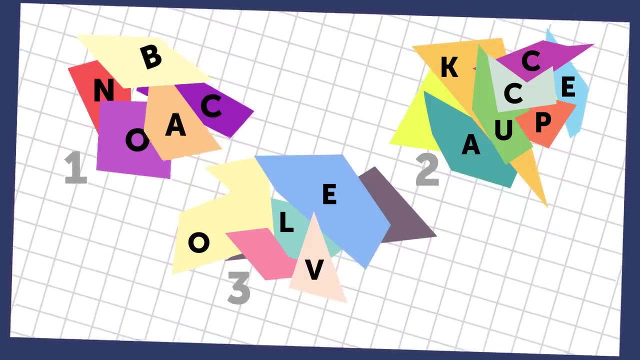 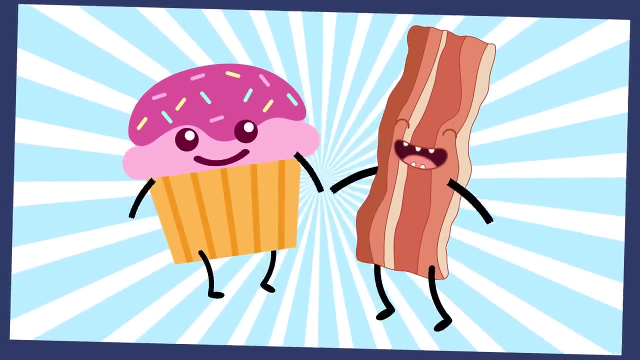 three groups of letters forms a word. Can you find out what the words are and find the odd one out? Think quickly, You have only 15 seconds. Let's look at it together. The first set of letters forms the word bacon. The second set makes the word cupcake- Ooh, bacon cupcakes. And the third. 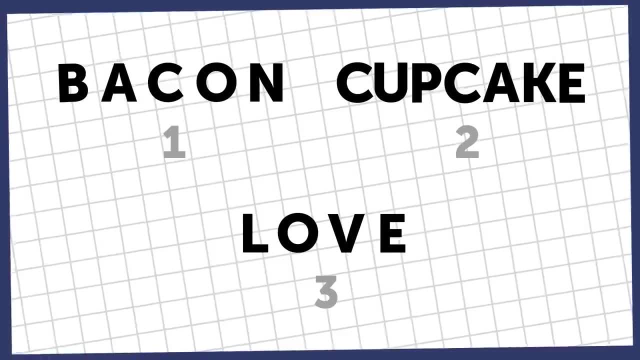 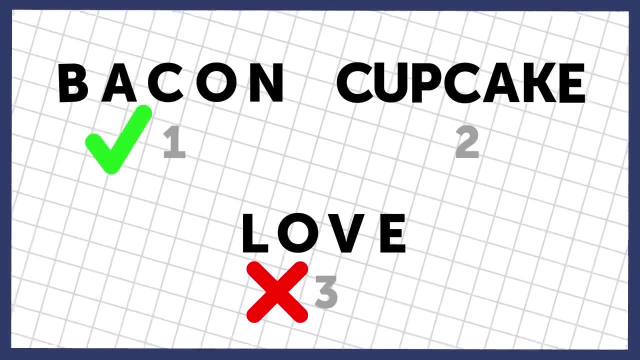 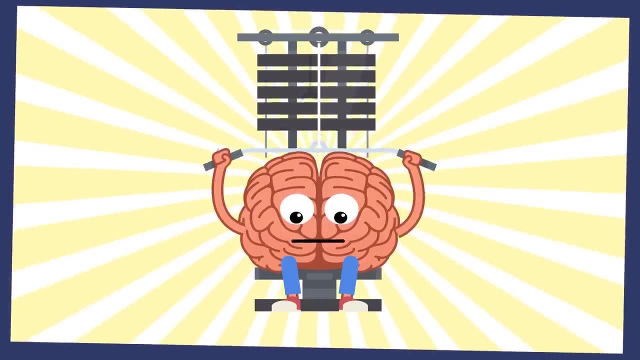 one says love. If you chose love as the odd one out, you're wrong. It's actually bacon, because cupcake and love both end with an E. We warned you that the riddles weren't easy, so keep an eye out. No, not literally, Don't take. 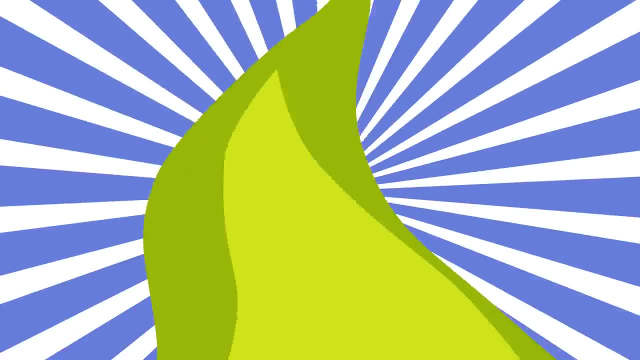 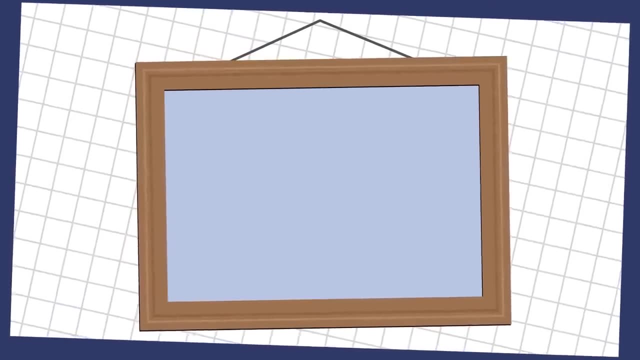 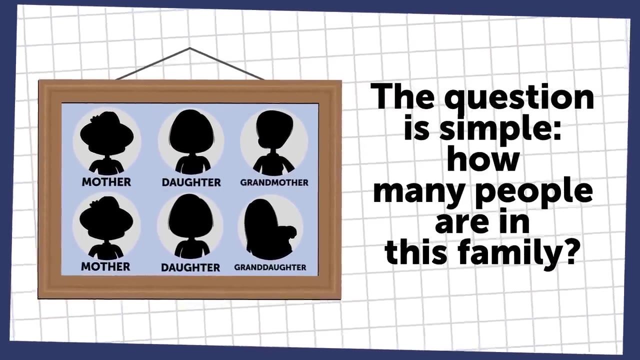 your eye out. Ew Riddle number three. Let's talk about family now. Imagine a family with two mothers, two daughters, one grandmother and one granddaughter. The question is simple: How many people are in this family? Count them all in 15 seconds. 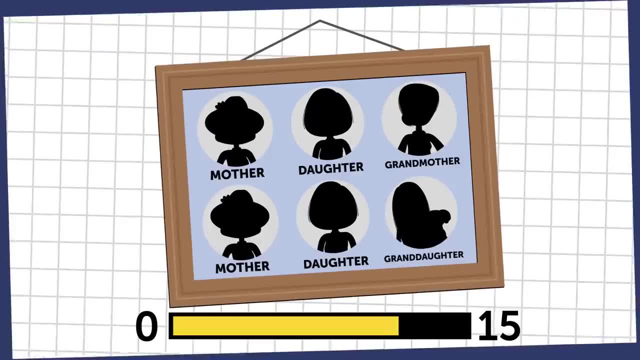 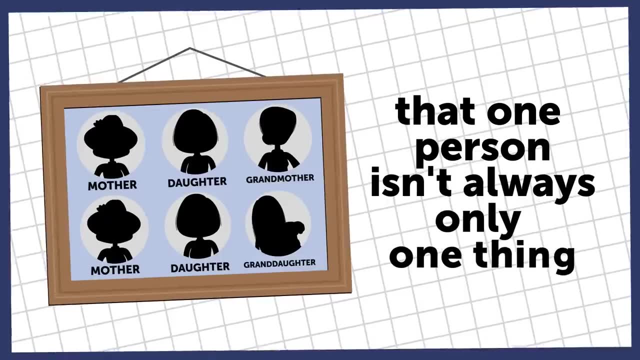 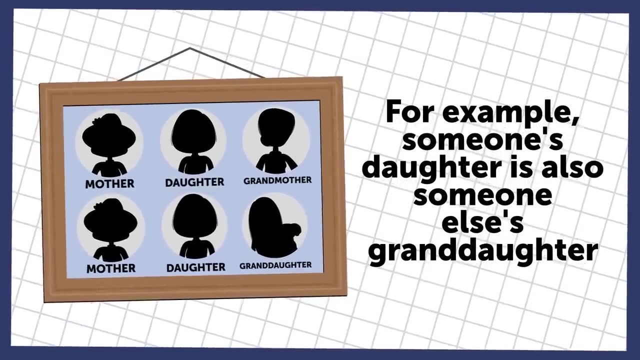 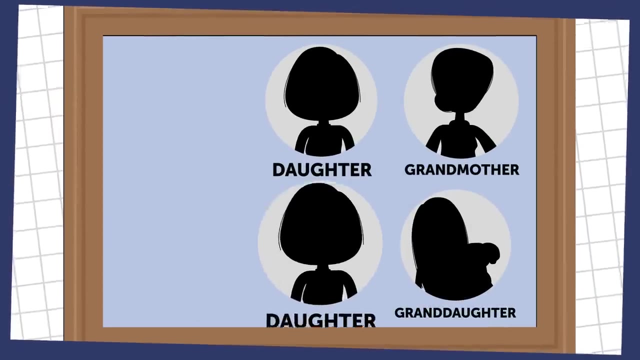 The key to cracking this riddle is remembering that one person isn't always only one thing. For example, someone's daughter is also someone else's granddaughter. In this particular family, there are actually three members: A grandmother, her daughter and her granddaughter. Think about: 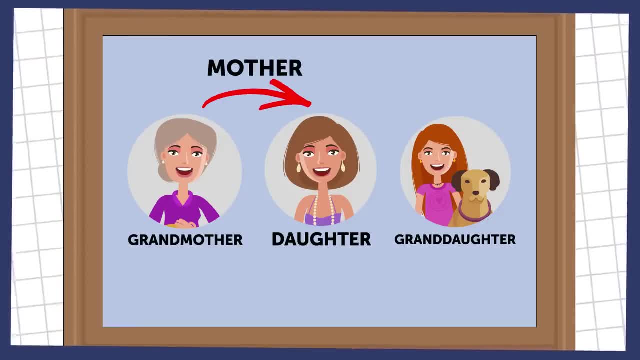 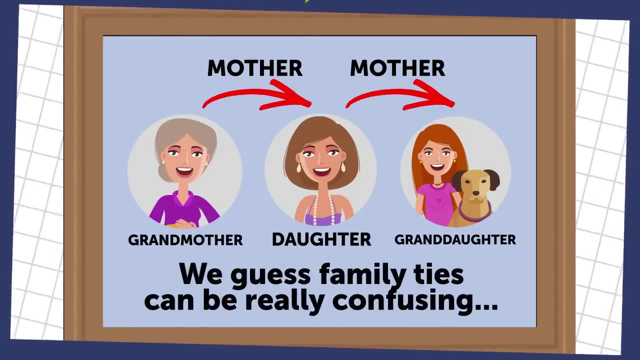 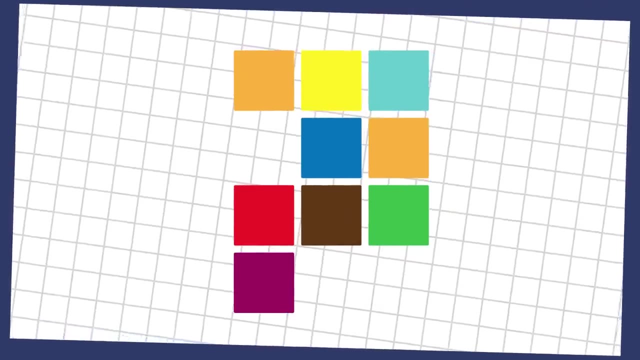 it. The grandmother is the mother to her daughter, The grandmother is the mother to her daughter daughter, while her daughter is the mother to her granddaughter. We guess family ties can be really confusing. Riddle number four: Look at this shape carefully. 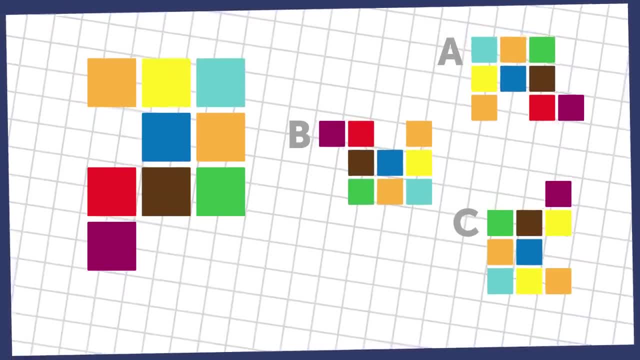 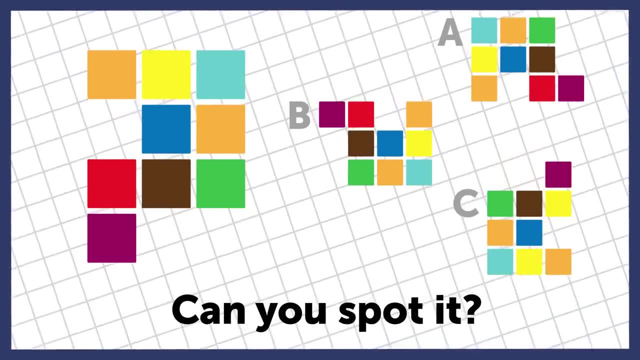 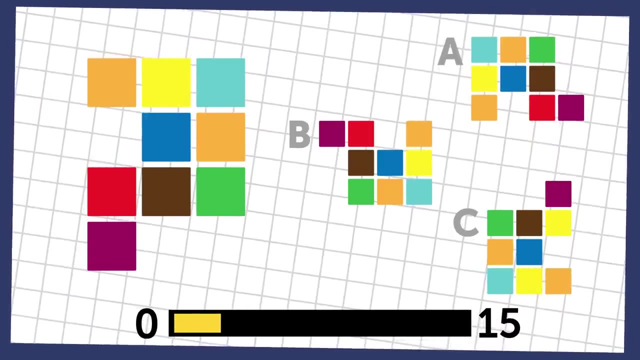 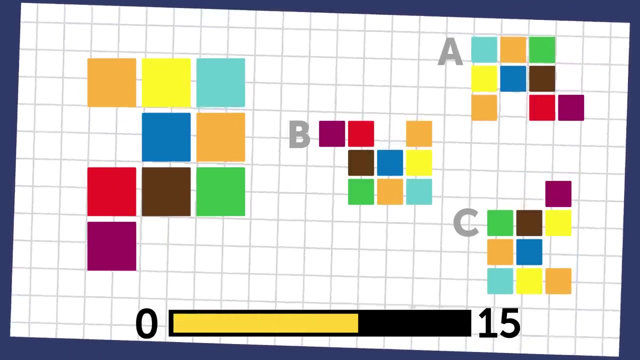 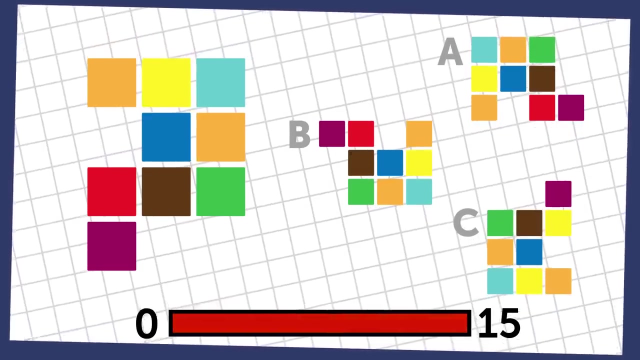 Now look at these three shapes that it becomes if you turn it to one side or the other. One of these three is again an odd one out. Can you spot it? Time is ticking. If you chose shape C as the odd one out, congratulations. 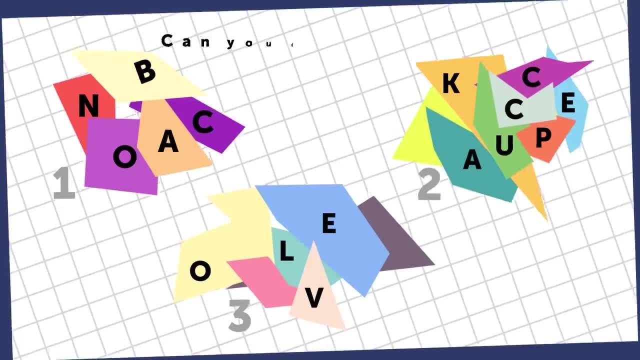 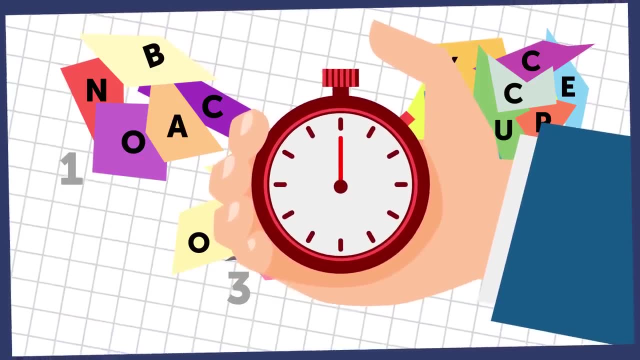 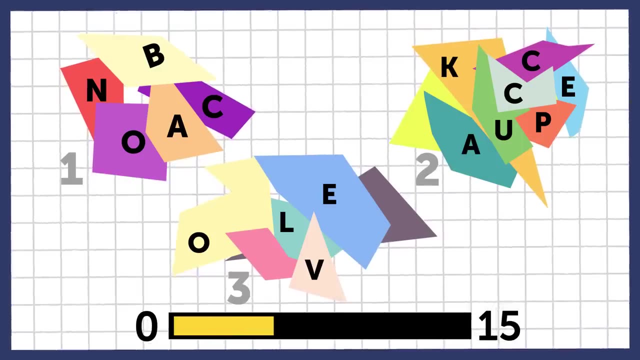 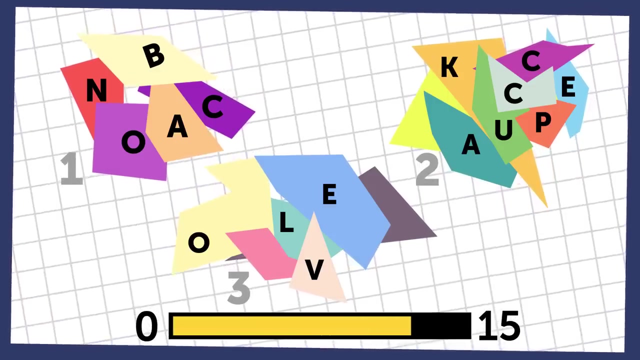 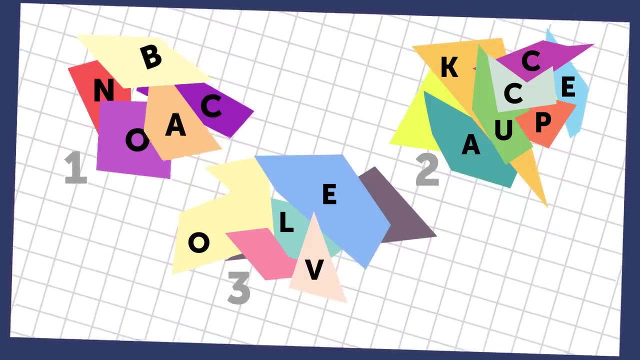 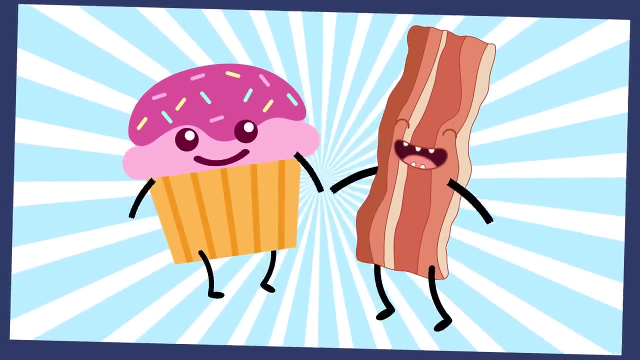 three groups of letters forms a word. Can you find out what the words are and find the odd one out? Think quickly, You have only 15 seconds. Let's look at it together. The first set of letters forms the word bacon. The second set makes the word cupcake- Ooh, bacon cupcakes. And the third. 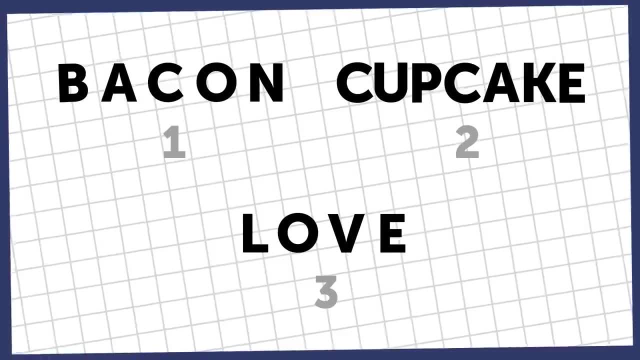 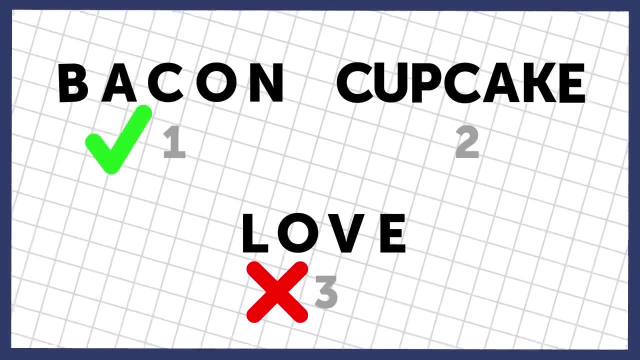 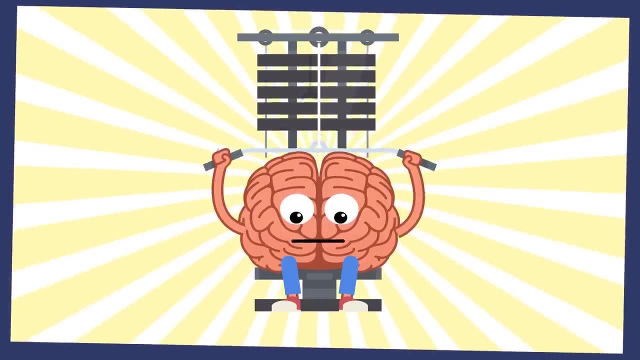 one says love. If you chose love as the odd one out, you're wrong. It's actually bacon, because cupcake and love both end with an E. We warned you that the riddles weren't easy, so keep an eye out. No, not literally, Don't take. 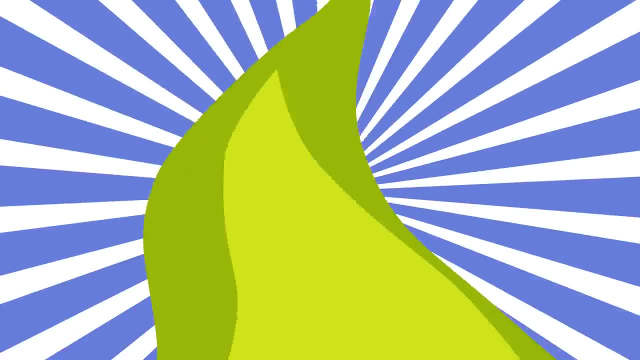 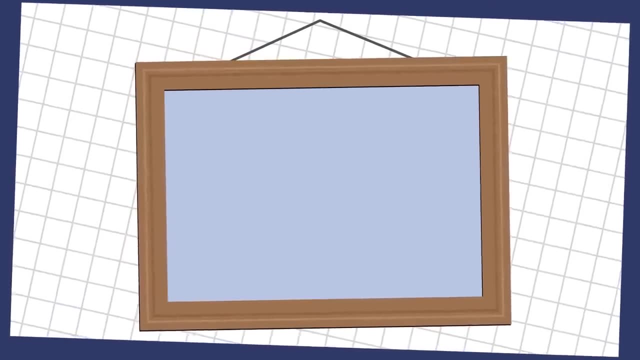 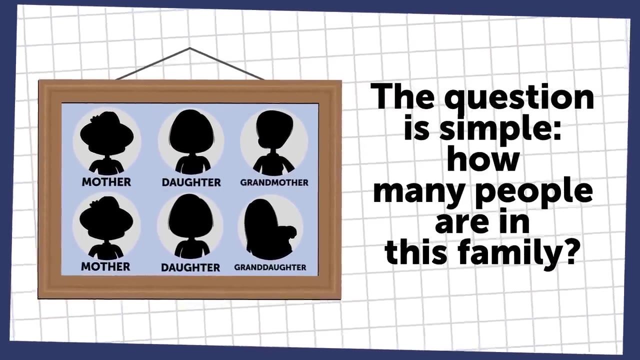 your eye out. Ew Riddle number three. Let's talk about family now. Imagine a family with two mothers, two daughters, one grandmother and one granddaughter. The question is simple: How many people are in this family? Count them all in 15 seconds. 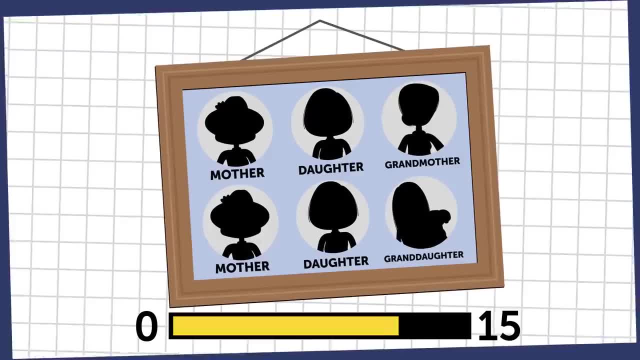 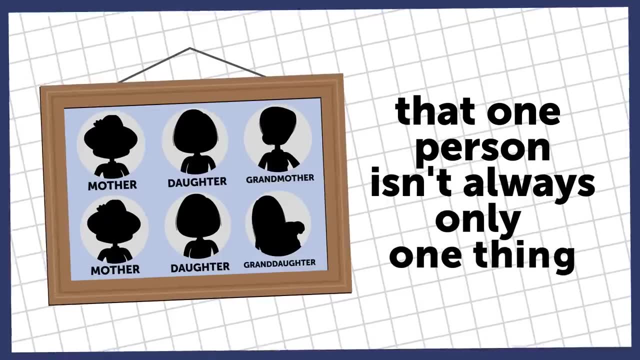 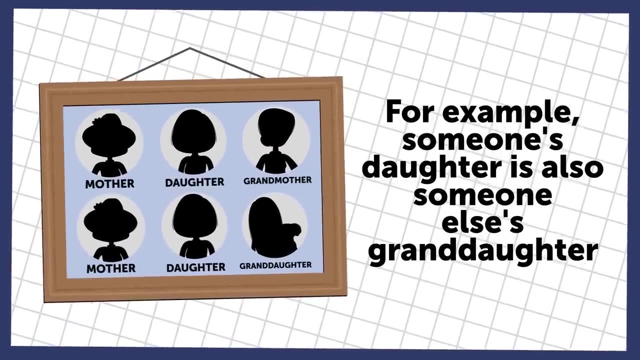 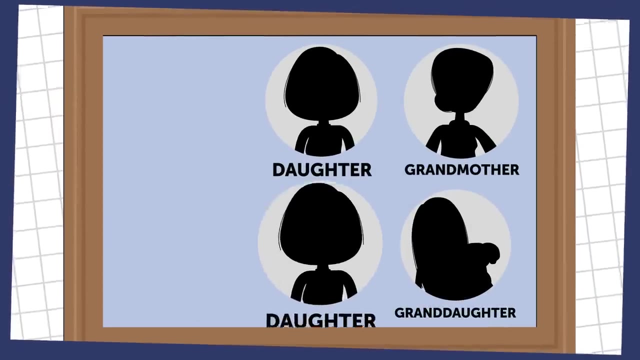 pless To crack at this riddle. You have to remember that one person isn't always one thing. For example, someone's daughter is also someone else's granddaughter. In this particular family, there are actually three members — a grandmother, her daughter and her granddaughter. Think about it: The grandmother is the mother to her daughter. 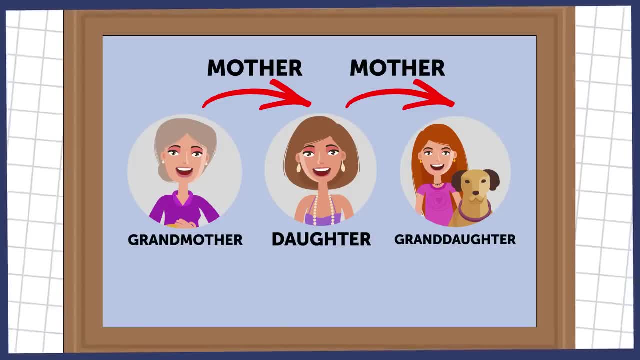 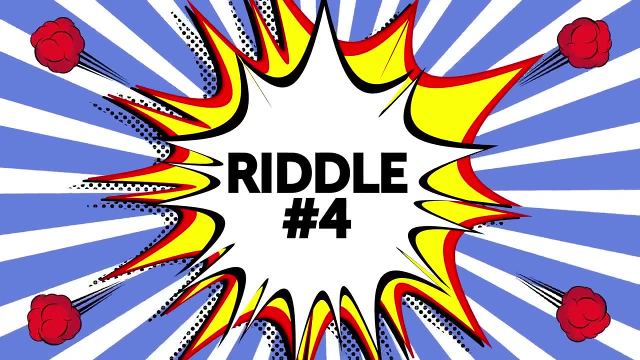 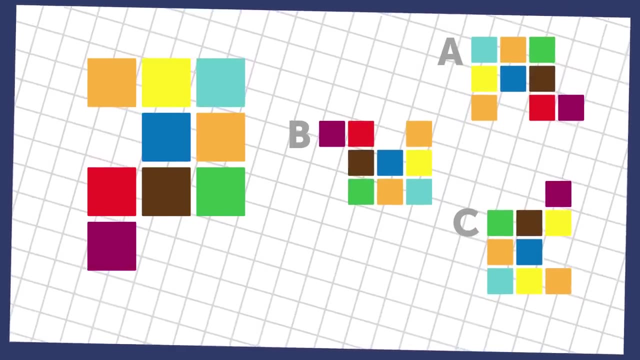 while her daughter is the mother to her granddaughter. We guess family ties can be really confusing. Riddle number four: Look at this shape carefully. Now look at these three shapes that it becomes if you turn it to one side or the other. 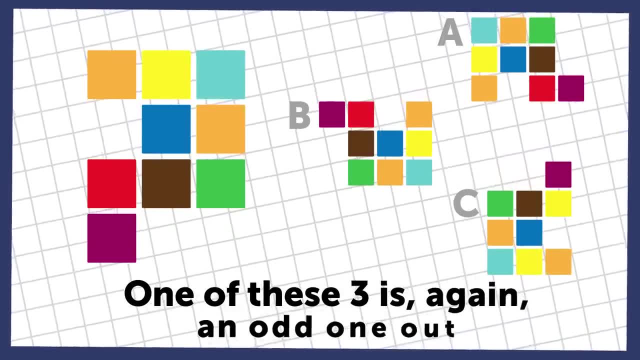 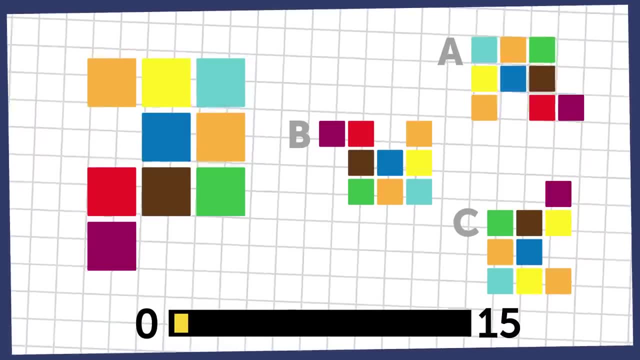 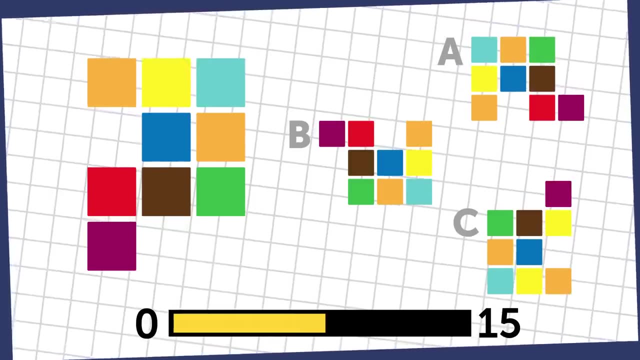 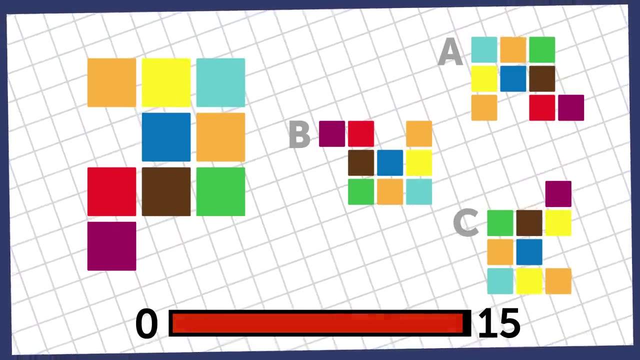 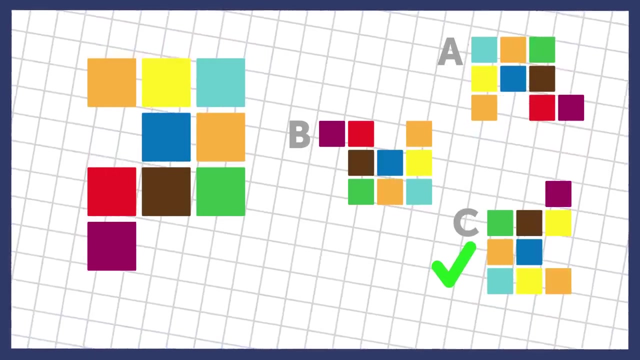 One of these three is again an odd one out. Can you spot it? Time is ticking. Click. If you chose shape C as the odd one out, congratulations, You've passed this task. Look at it once again: The red square here at the end. 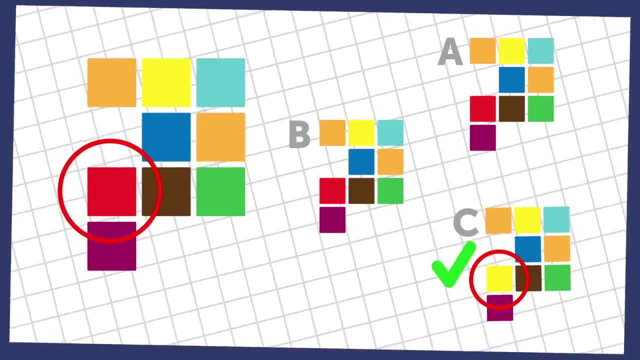 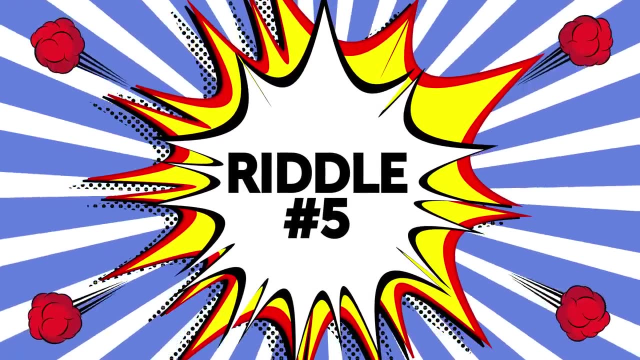 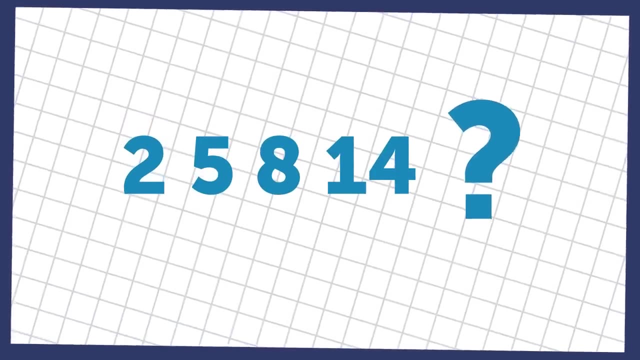 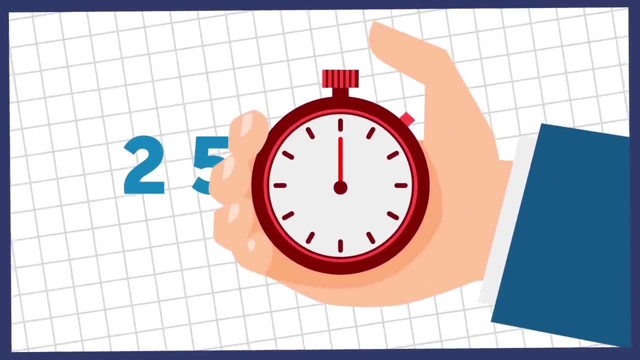 is missing, while shapes A and B are perfectly fine. Attention is the key Riddle number five, Two, five, eight, fourteen. and Can you figure out what the next number should be and why? Time to use your logical thinking again. 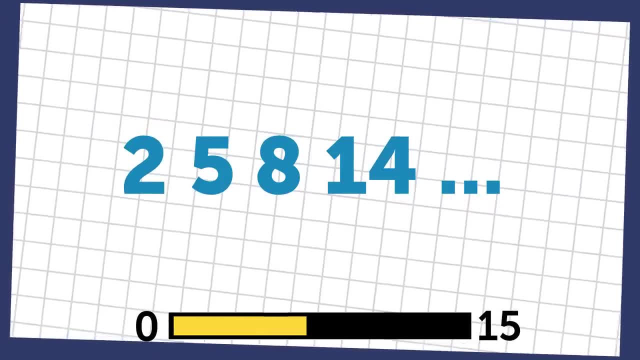 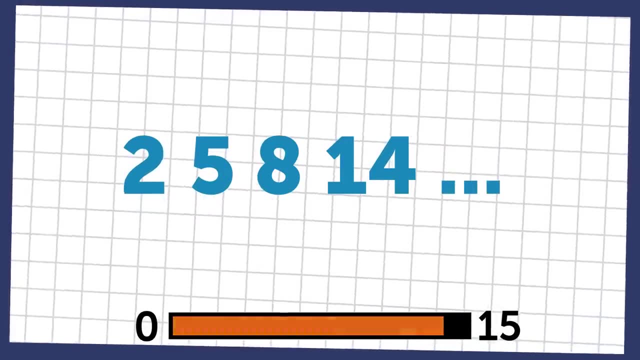 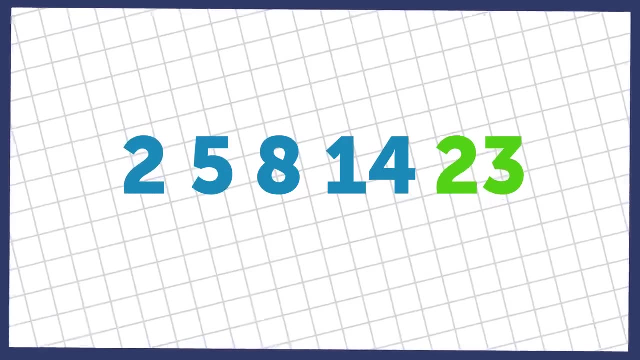 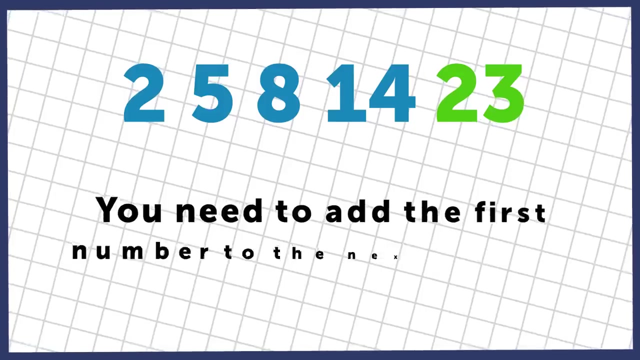 The correct answer here is twenty-three. Did you guess correctly? The pattern is very simple. You need to add the first number to the next number and add one after that. For example, two plus five is seven and seven plus one is eight. 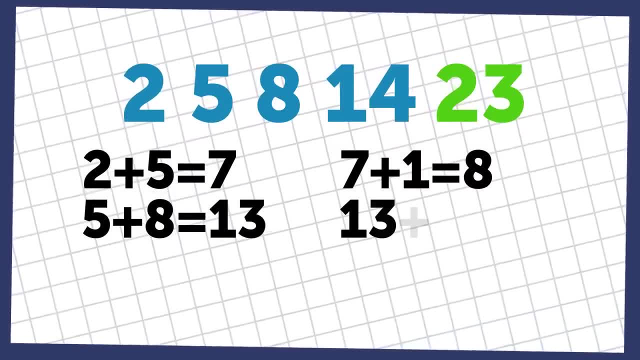 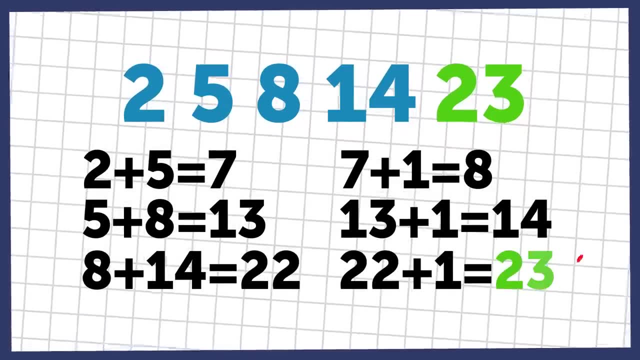 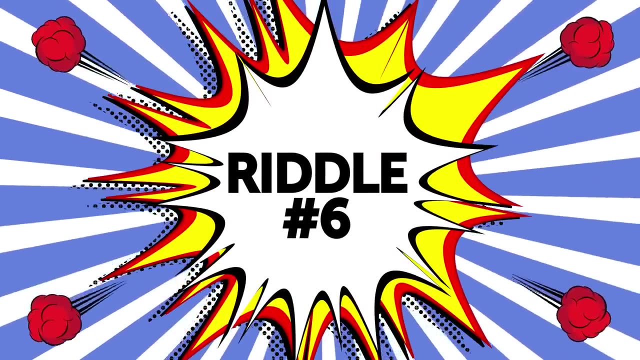 Then five plus eight is thirteen, and thirteen plus one is fourteen, And finally, eight plus fourteen is twenty-two, and twenty-two plus one is twenty-three. Eh, just like that Riddle number six. Look at these four letter combinations. 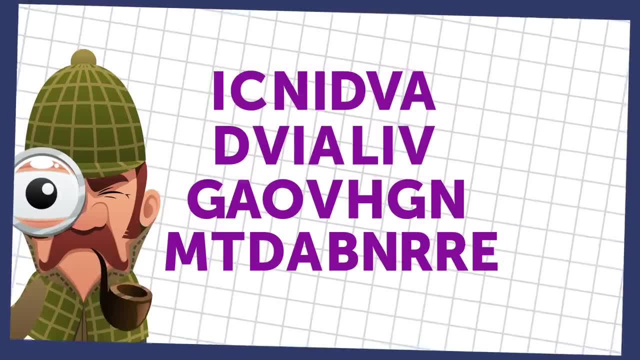 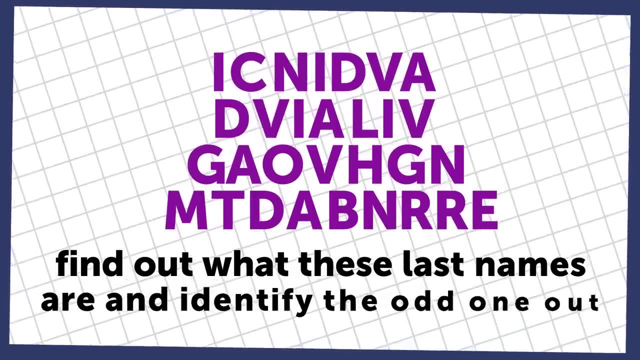 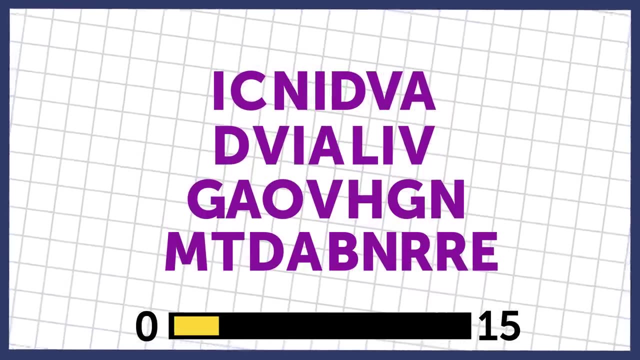 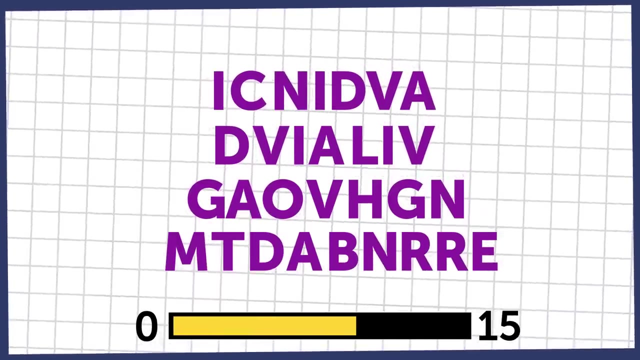 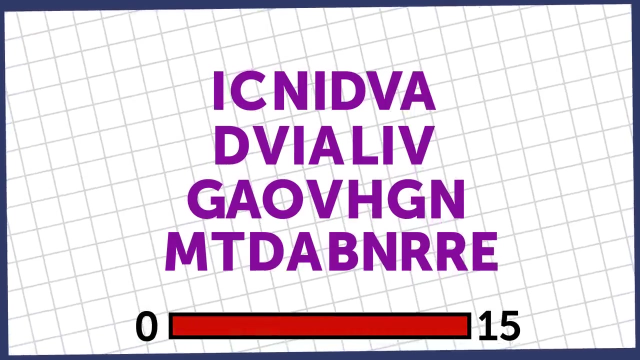 Each of them forms the last name of a famous person. Your task is simple: Find out what these last names are and identify the odd one out. Your fifteen seconds start now. Well, let's see whether you cracked this riddle. The first name is Da Vinci. 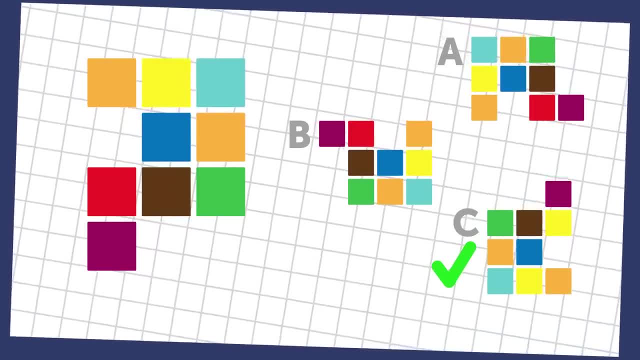 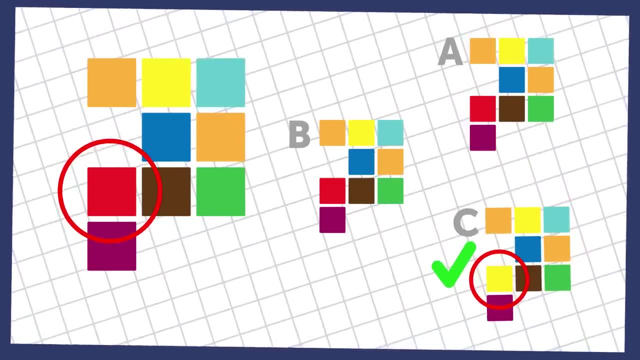 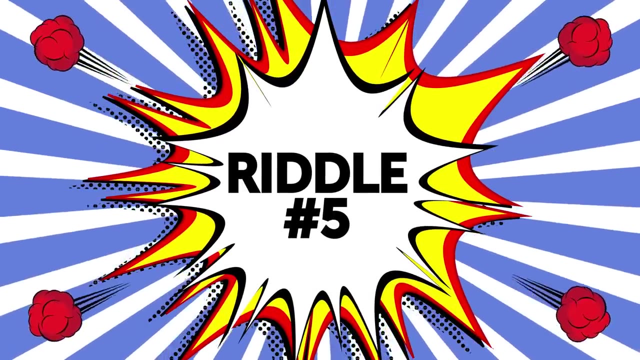 You've passed this task. Look at it once again. The red square here at the end is missing, while shapes A and B are perfectly fine. Attention is the key Riddle. number five, Two, five, eight, fourteen and…. 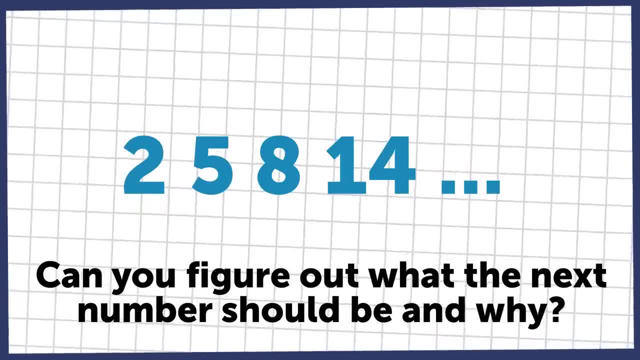 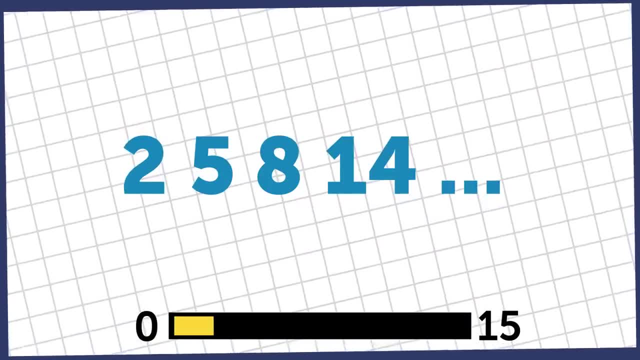 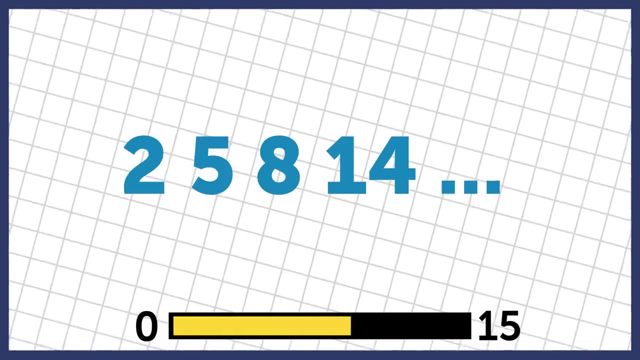 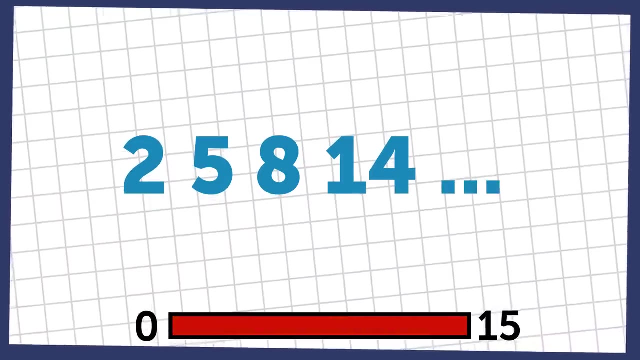 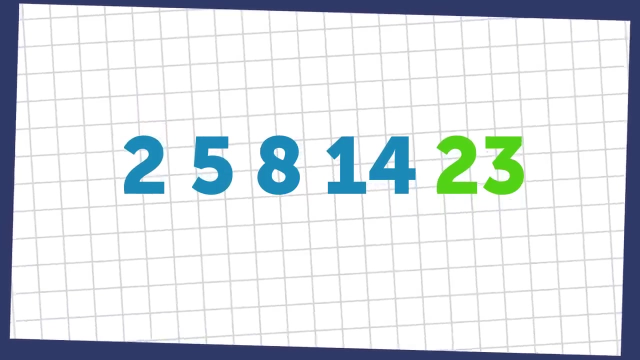 Can you figure out what the next number should be and why? Time to use your logical thinking again. I'm sorry. I'm sorry. The correct answer here is twenty-three. Did you guess correctly? The pattern is very simple. You need to add the first number to the next number and add one after that. 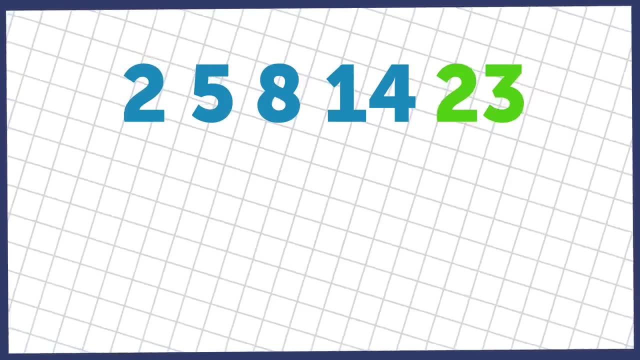 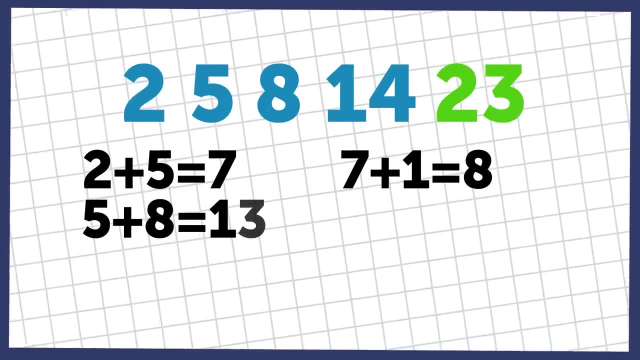 For example, two plus five is seven, and seven plus eight is twenty-three. Well, that's enough. Go on 5.. 7 plus 1 is 8, then 5 plus 8 is 13,, and 13 plus 1 is 14.. 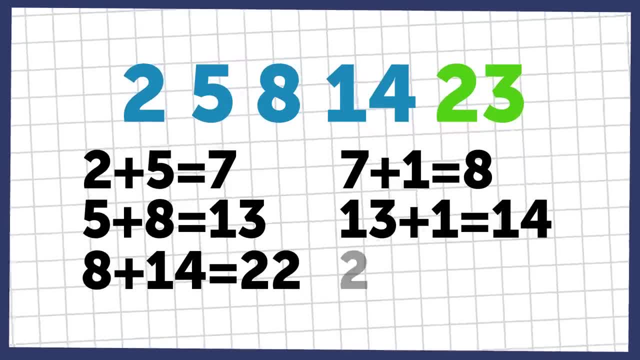 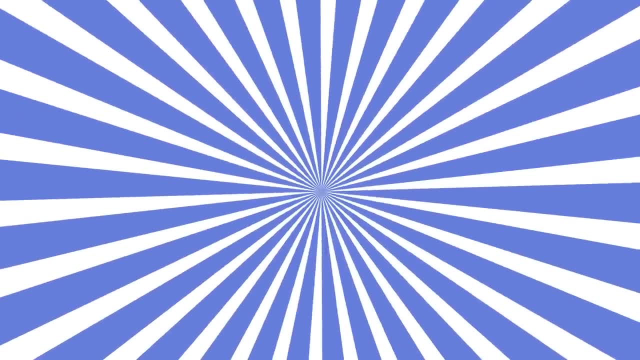 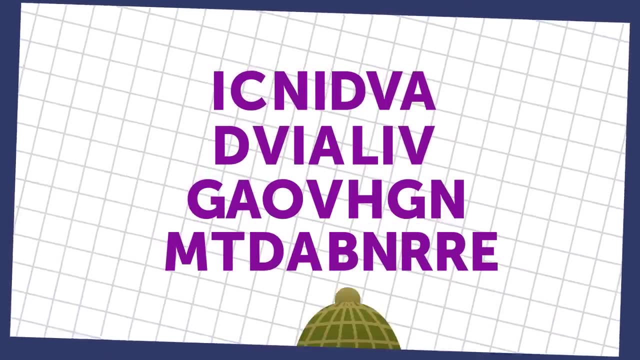 And finally, 8 plus 14 is 22,, and 22 plus 1 is 23.. Eh, just like that Riddle number 6.. Look at these four letter combinations. Each of them forms the last name of a famous person. 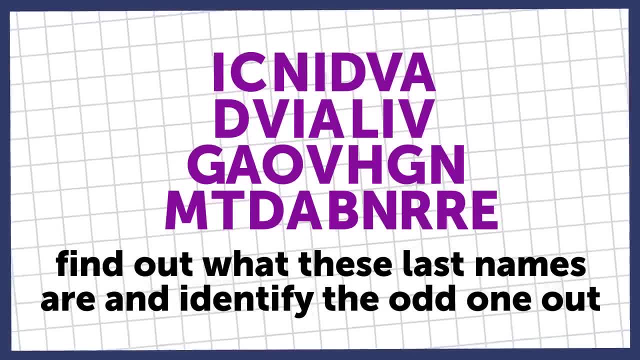 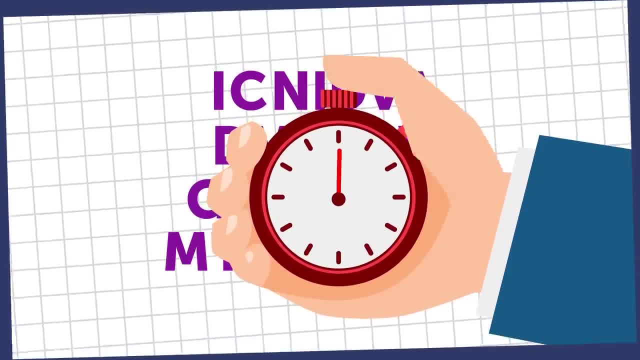 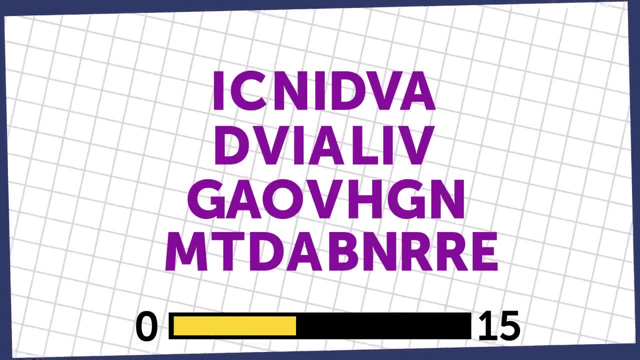 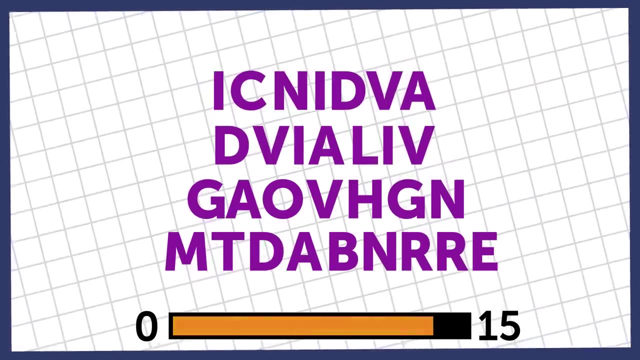 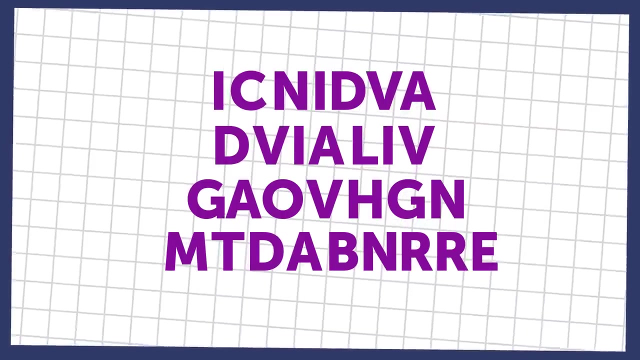 Your task is simple: Find out what these last names are and identify the odd one out. Your 15 seconds start now. Well, let's see whether you cracked this riddle. The first name is Da Vinci, The second one is Vivaldi. 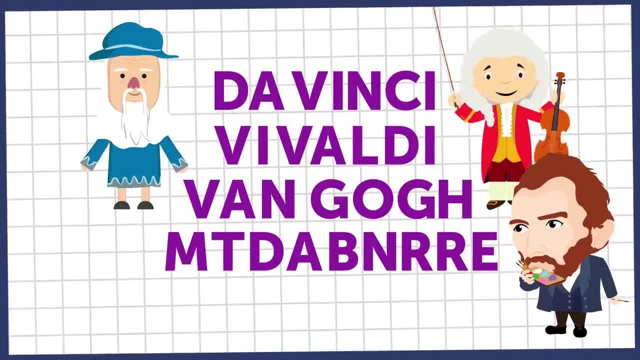 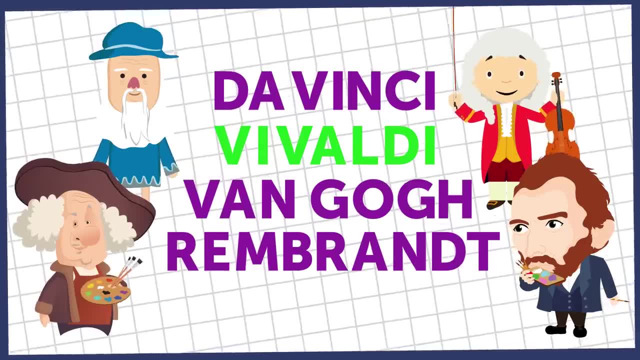 The third one is Van Gogh And the final one is Rembrandt. If you've answered this part right, you've probably picked Vivaldi as the odd one out, which is right. He's the only composer in this list of painters. 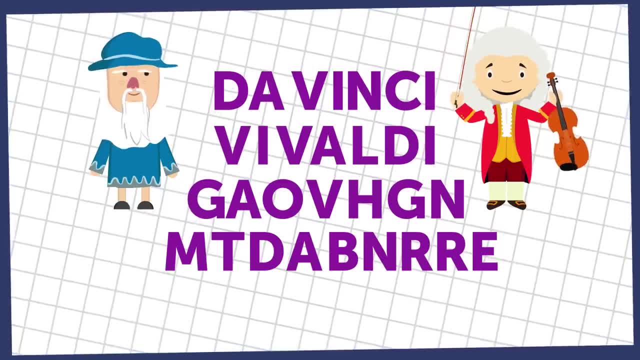 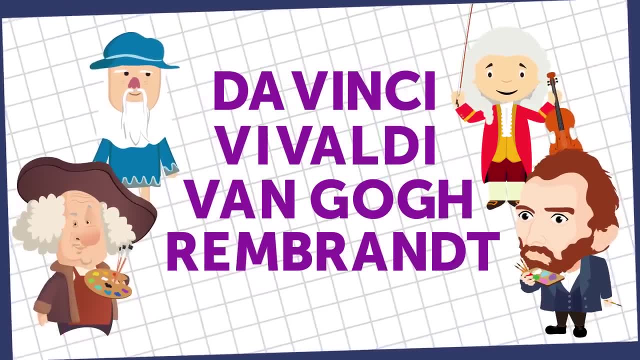 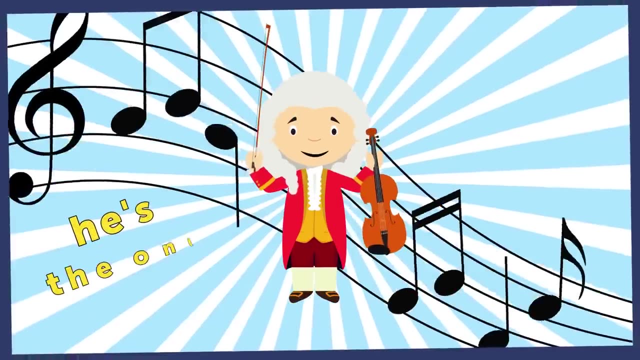 The second one is Vivaldi, The third one is Van Gogh And the final one is Rembrandt. If you've answered this part right, you've probably picked Vivaldi as the odd one out, which is right. He's the only composer in this list of painters. 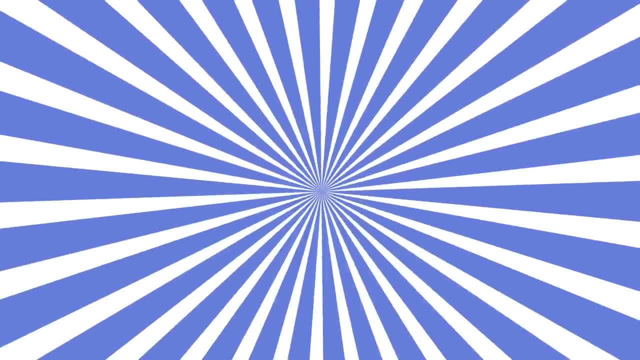 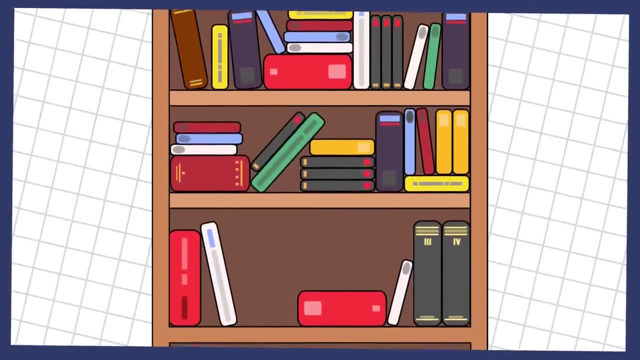 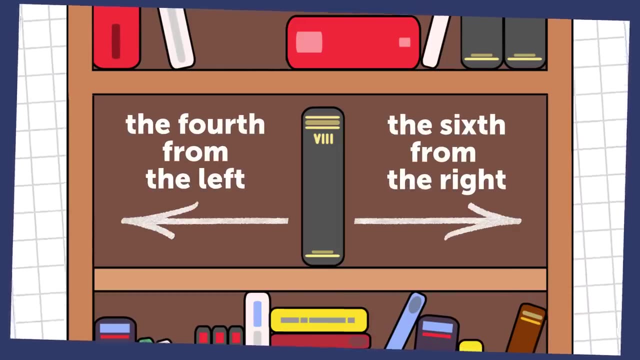 Well done, Riddle number seven. There's a shelf of books in a library. On this shelf, a particular book is fourth from the left and the sixth from the right. Knowing this, can you figure out how many books there are on this shelf? 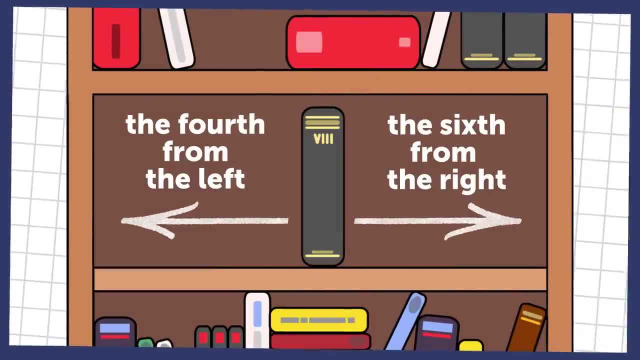 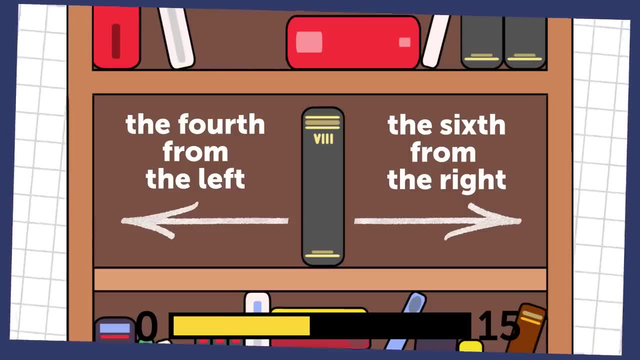 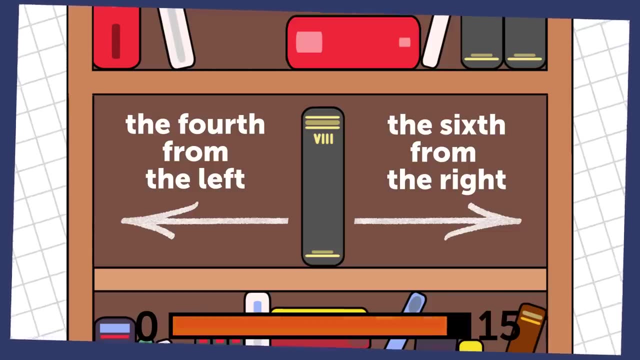 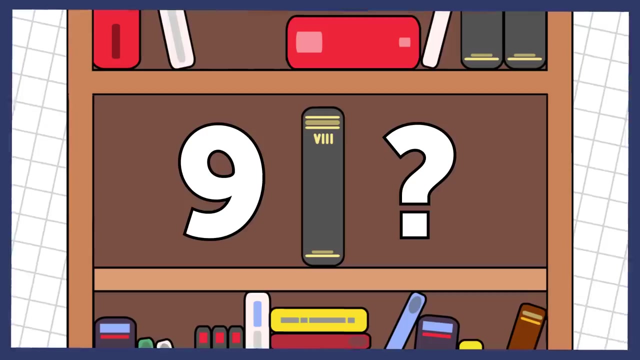 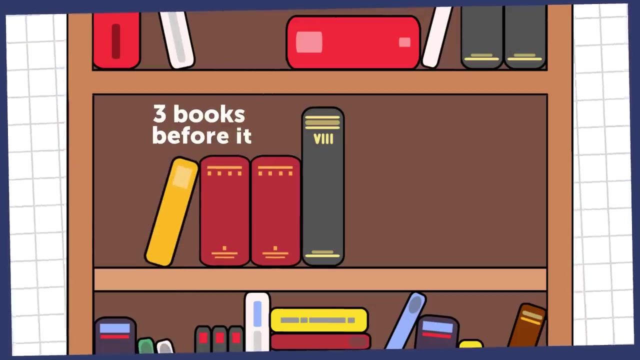 Tick-tock. If your answer is nine, you're right and should give yourself a pat on the back if your arm's long enough. If the book is the fourth from the left, that means there are three books before it, And if it's the sixth from the right, that means there are five books after it. 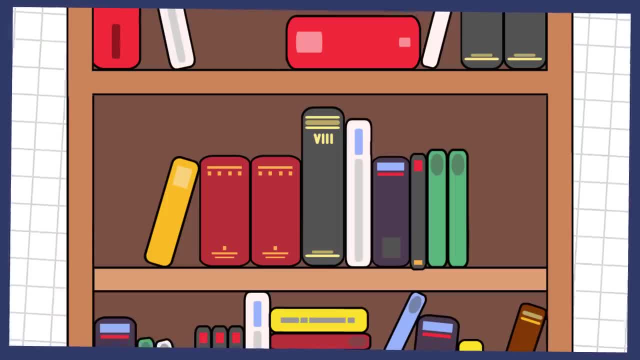 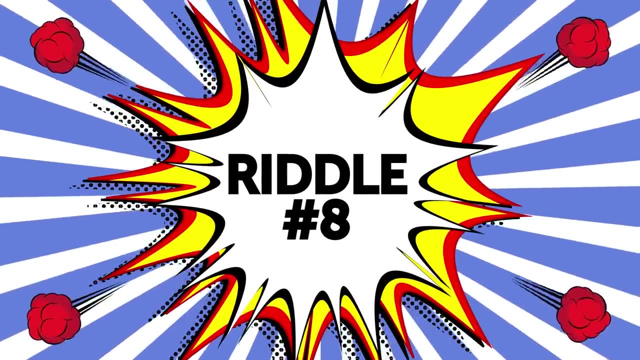 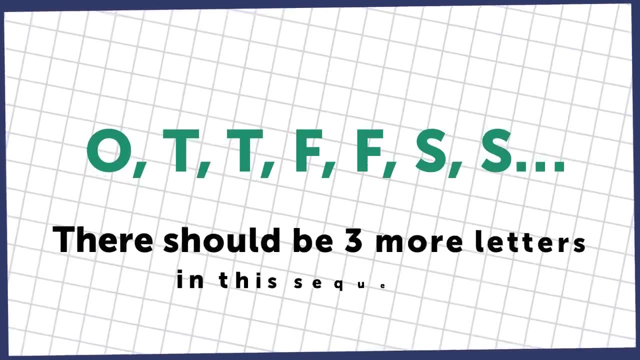 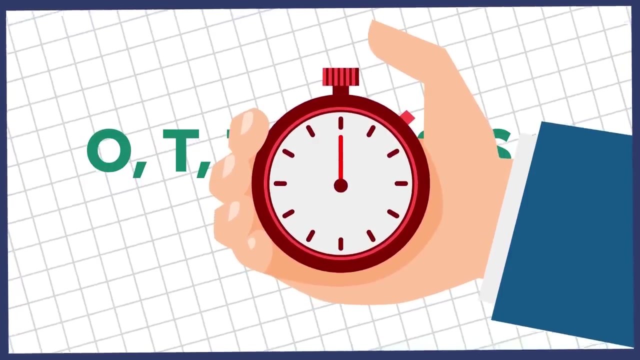 Five plus three is eight, plus the book itself gives us nine. Riddle number eight: O-T-T-F-F-S-S. There should be three more letters in this sequence, but what are they? Use these 15 seconds to crack this riddle. 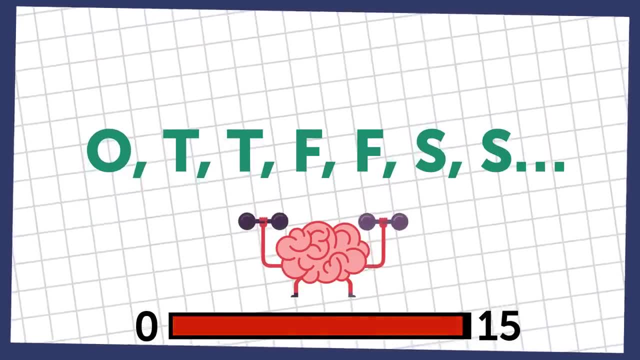 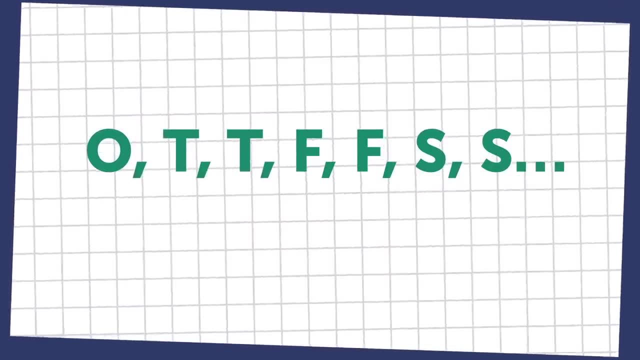 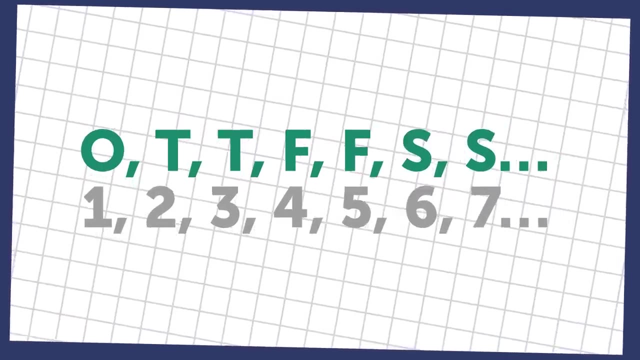 The correct answer is much simpler and easier than you probably thought. These numbers represent the first letters of the numbers 1 to 10.. Here we finished on a 7, so the next three letters are E for 8,, N for 9, and T for 10.. 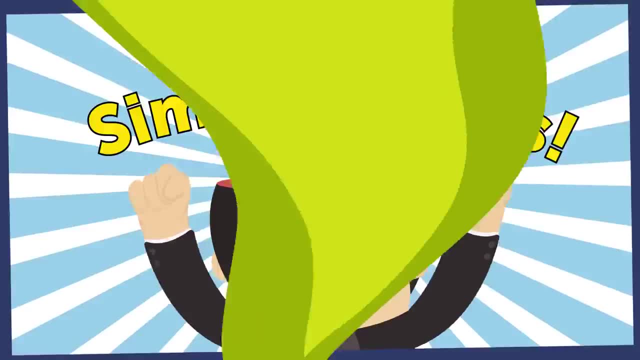 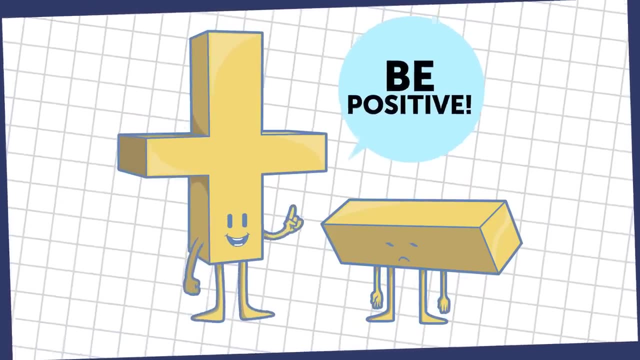 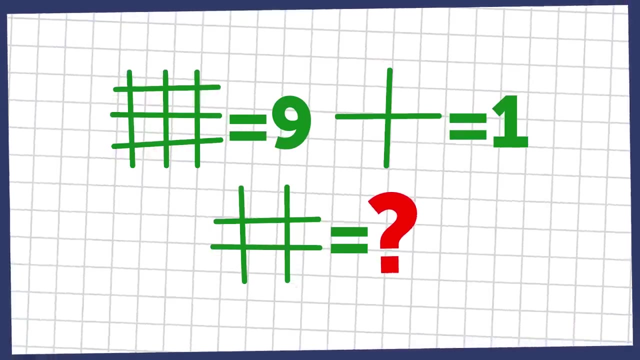 Simply genius: Riddle number nine. Let's throw a bit more math into the mix, shall we? Let's look at these two equations. Given this information, do you have any idea which number should be in the place of this question mark, and why? 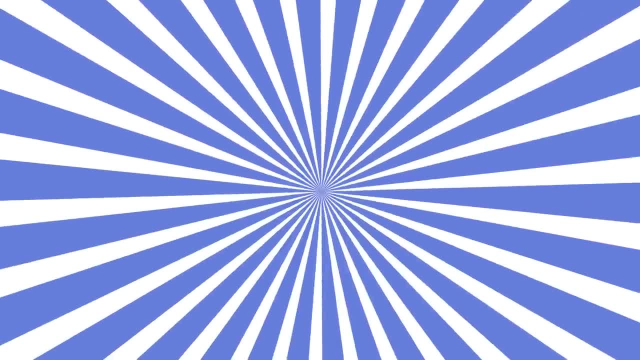 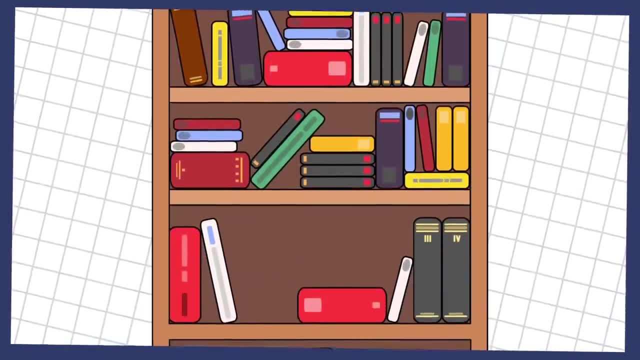 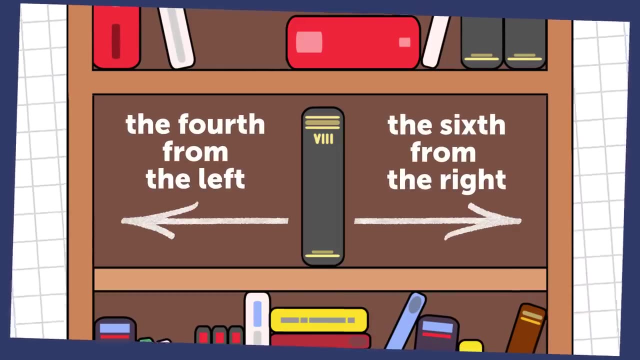 Well done. Riddle number 7.. Riddle number 7.. There's a shelf of books in a library. On this shelf, a particular book is fourth from the left and the sixth from the right. Knowing this, can you figure out how many books there are on this shelf? 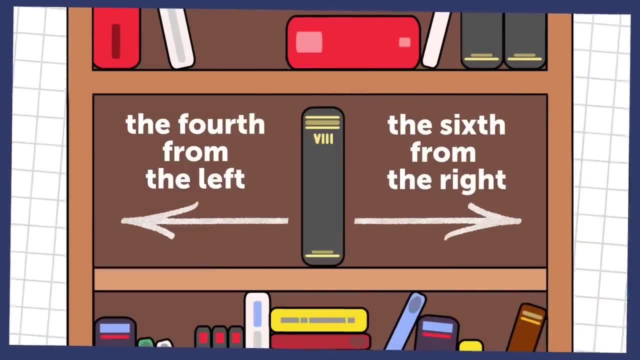 Tick-tock. Riddle number 8.. Riddle number 9.. Riddle number 10.. Riddle number 11.. Riddle number 12.. Riddle number 13.. Riddle number 14.. Riddle number 15.. 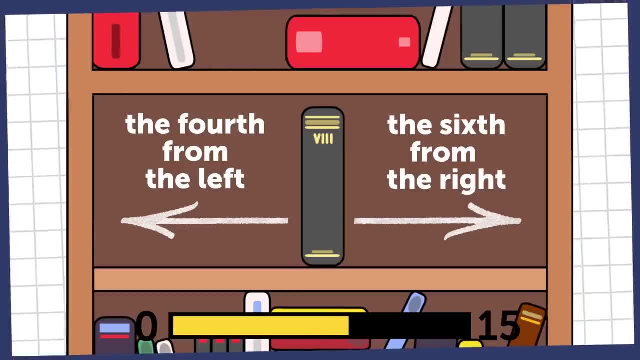 Riddle number 16.. Riddle number 17.. Riddle number 18.. Riddle number 19.. Riddle number 19.. Riddle number 20.. Riddle number 21.. R into ute Riddle number 22.. 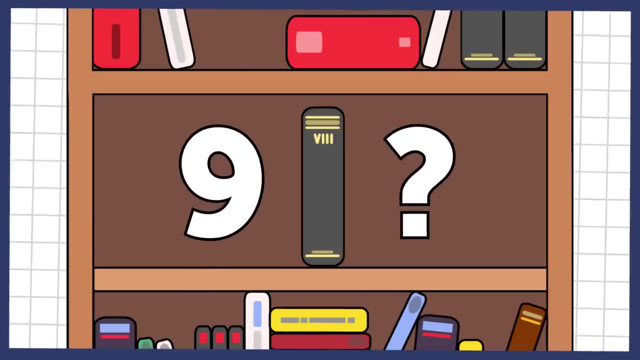 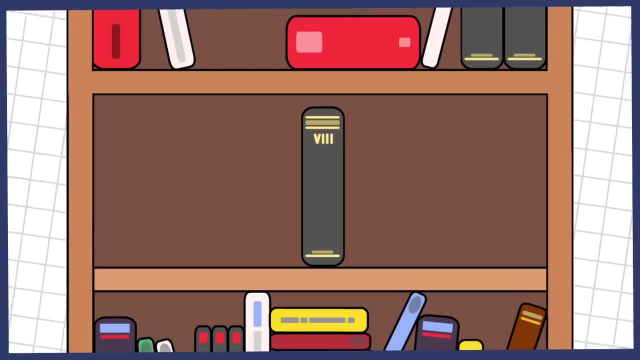 R into ust in st place shining subscribe. If your answer is 9,, you're right and should give yourself a pat on the back if your arm's long enough. If the book is the 4th from the left, that means there are 3 books before it. 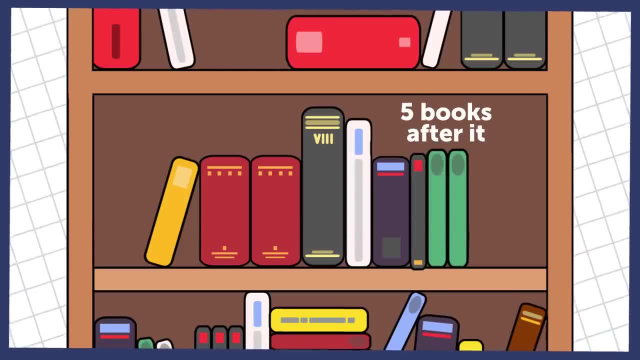 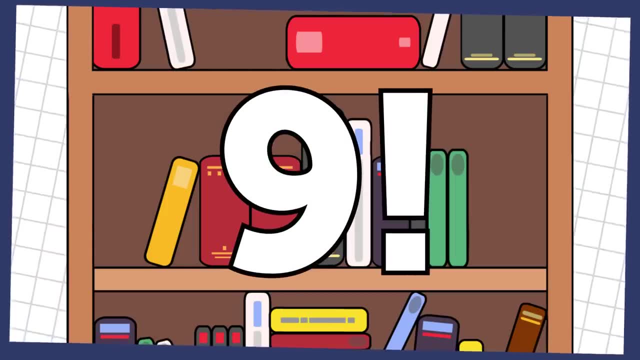 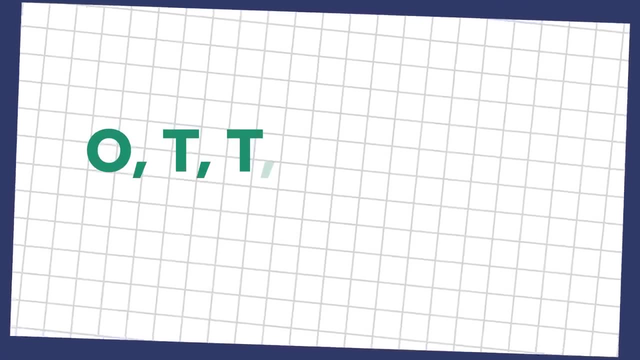 And if it's the 6th from the right, that means there are 5 books after it. 5 plus 3 is 8, plus the book itself gives us 9.. Riddle number eight: O-T-T-F-F-S-S. 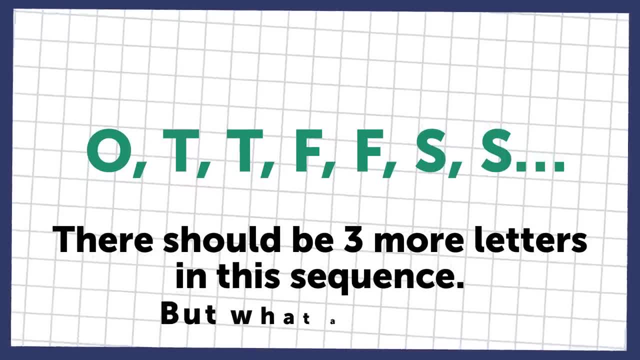 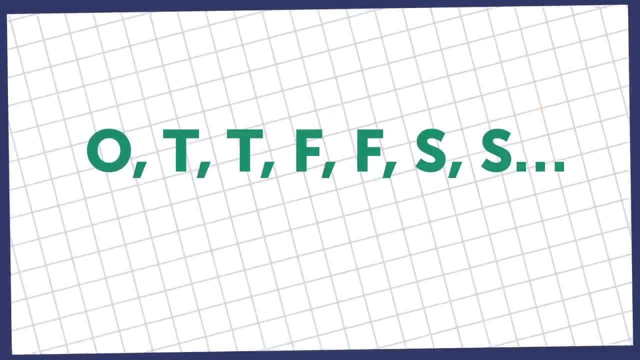 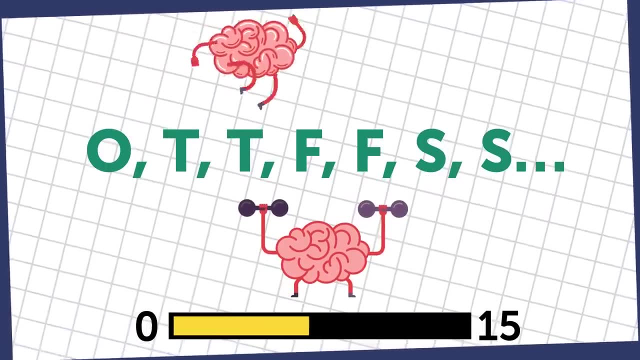 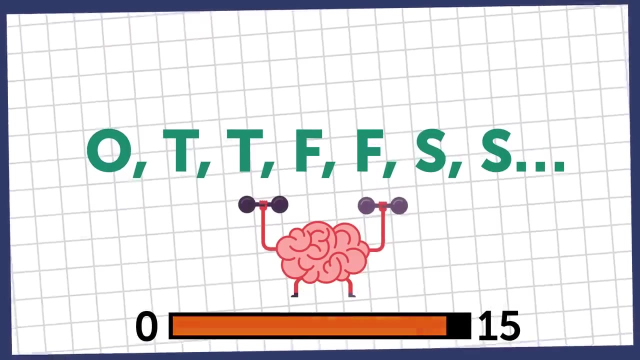 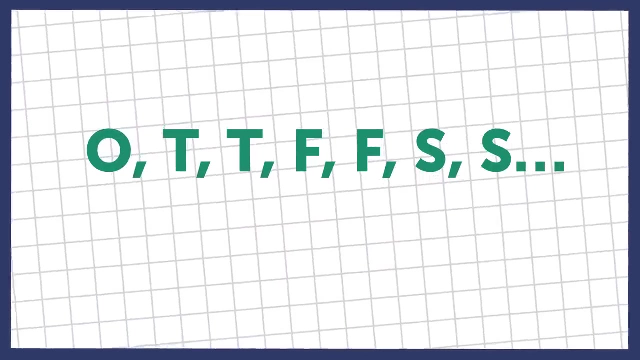 There should be three more letters in this sequence, But what are they? Use these 15 seconds to crack this riddle. The correct answer is much simpler and easier than you probably thought. These numbers represent the first letters of the numbers 1 to 10.. 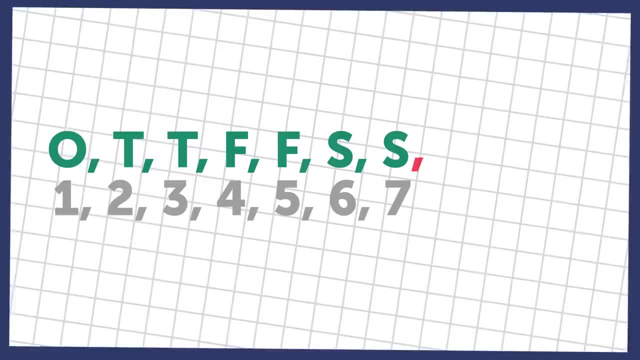 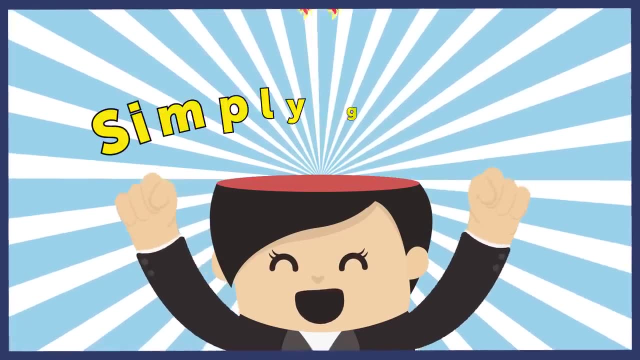 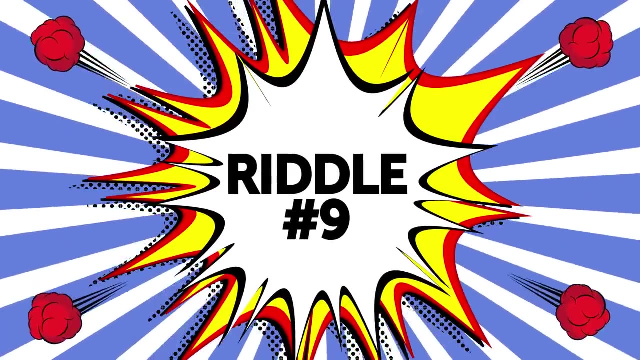 Here we finished on a 7.. So the next three letters are E for 8,, N for 9, and T for 10.. Simply genius, RIDDLE NUMBER NINE. Let's throw a bit more math into the mix, shall we?